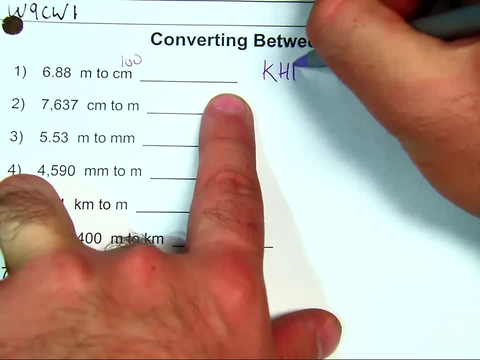 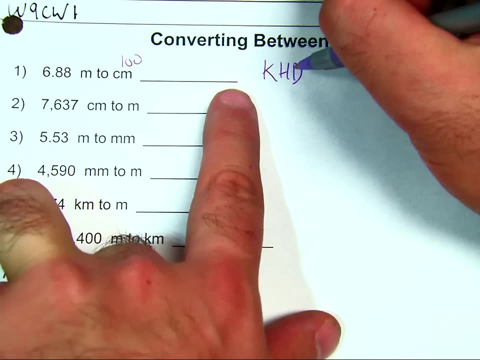 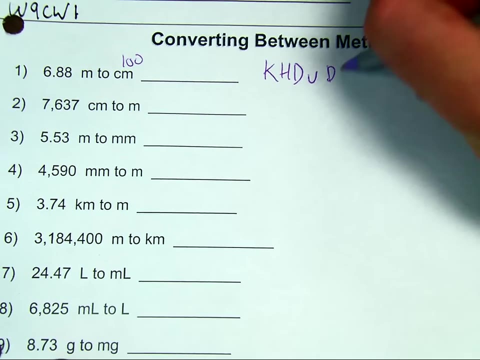 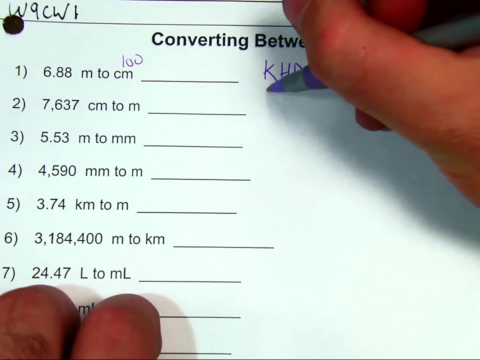 The science teacher showed me this, It goes. King Henry died unexpectedly drinking chocolate milk. Sorry about that. King Henry died unexpectedly drinking chocolate milk. This stands for kilometers, hectometers, decameters, your unit, which could be also M, G or L. 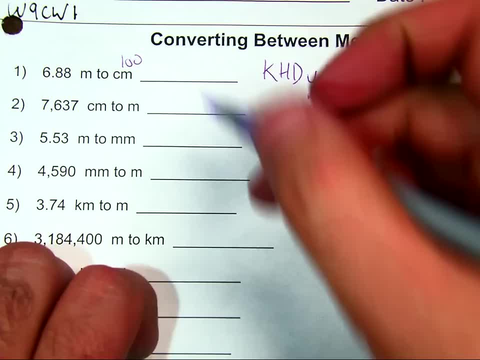 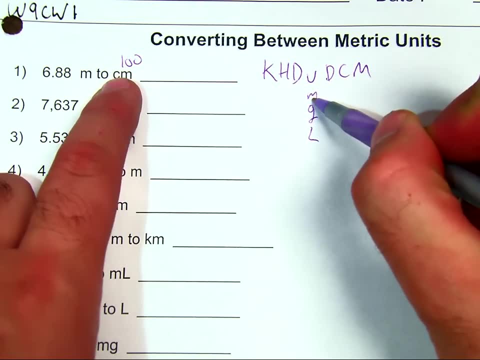 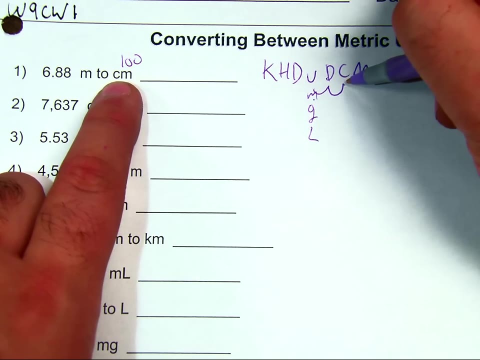 Decameters, centimeters or millimeters. So we're converting from meters to centimeters. So I'm going to count how many spaces I'm going to move over. I'm going one, two spaces from my M to my C. 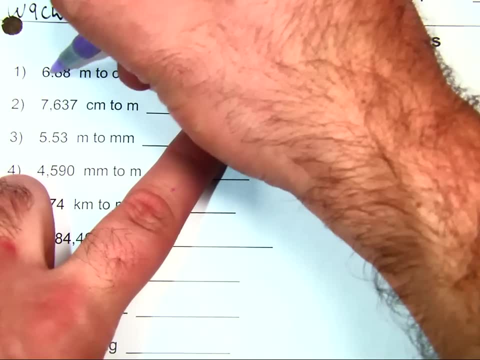 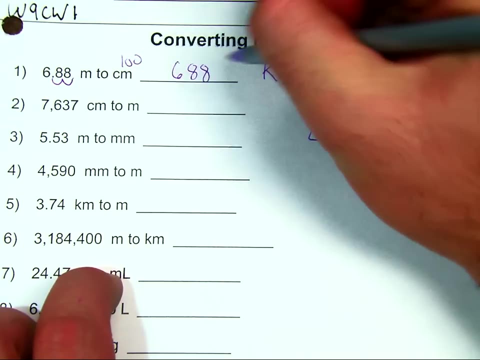 In this case, I'm going to move over two spaces to the right as well, Going one, two spaces to the right. So my final answer will be 688.. I'm going 2.588 centimeters. My next one I'm doing in block 10.. 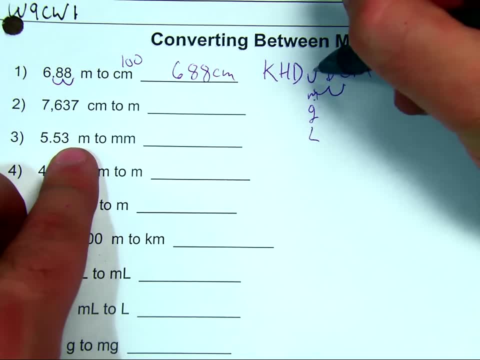 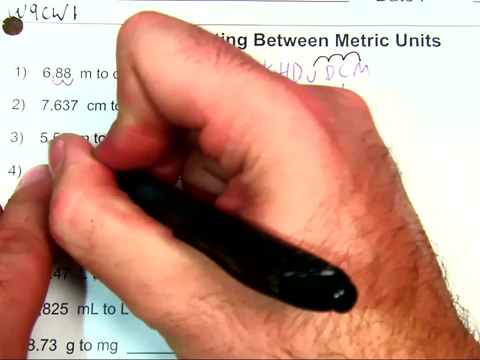 For my next one, I'm going- let's do number three- meters to millimeters. I'm going from my unit, my M, to my millimeter. I'm going one, two, three spaces to the right. So I'm gonna go one, two, three spaces to the right. 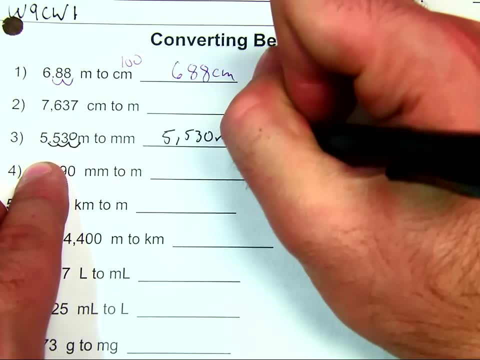 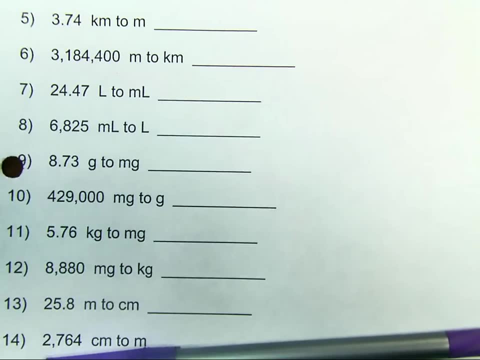 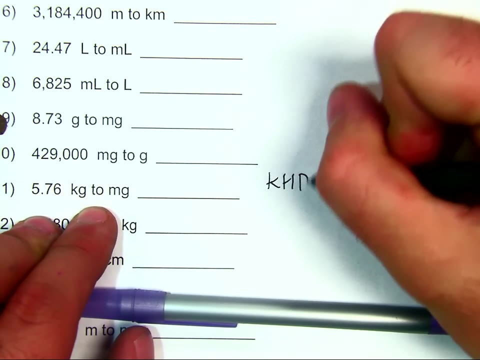 Now I ran out of space so I have to add a placeholder zero, 5,530 millimeters Now, something that's kind of ridiculous like number 11.. I have 5.76 kilograms to milligrams. I have King Henry died unexpectedly drinking chocolate milk. I'm going to go from kilograms. 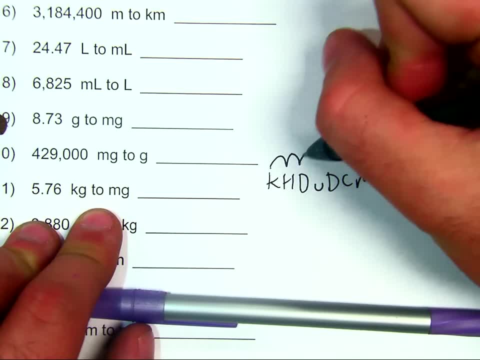 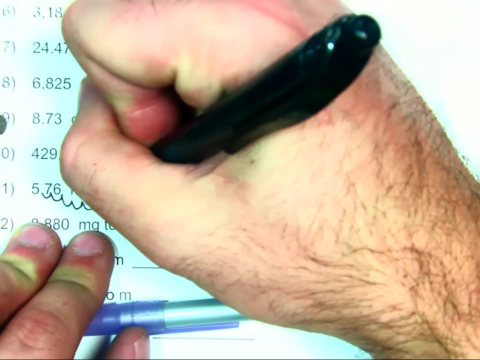 all the way to milligrams over here. So I'm going 1,, 2,, 3,, 4,, 5,, 6 spaces to the right. So I'm going to go 1,, 2,, 3,, 4,, 5,, 6 spaces to the right. I have 576.. And then 1,, 2,, 3,. 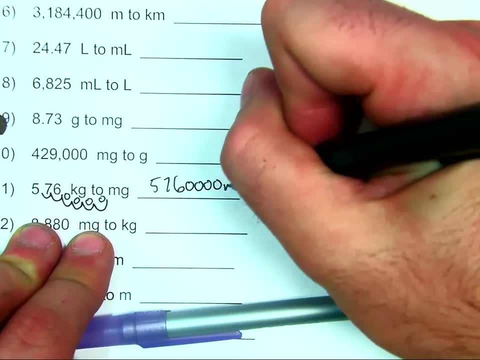 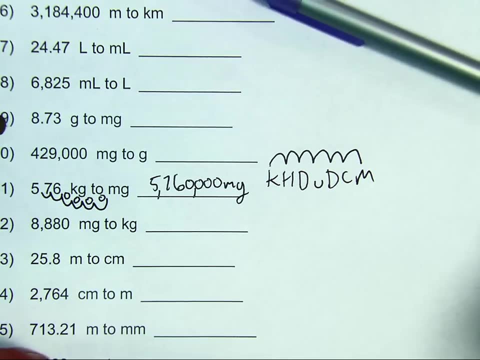 4 placeholder zeros. Now I add some commas to make sure it looks right. 5,760,000 milligrams. And one more: Let's just do our meters to centimeters right here, number 13.. 25.8 meters. 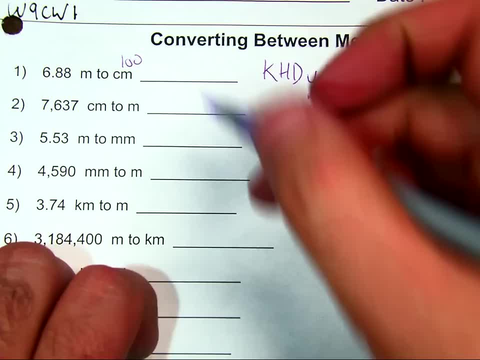 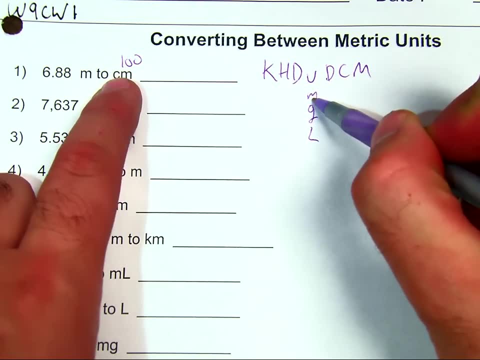 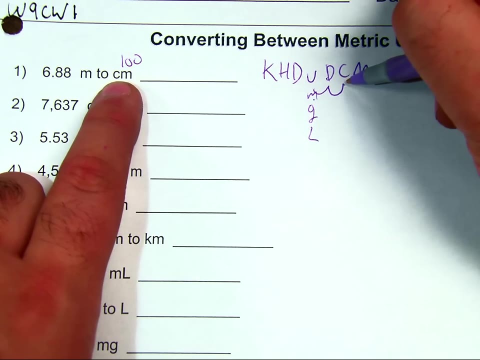 Decameters, centimeters or millimeters. So we're converting from meters to centimeters. So I'm going to count how many spaces I'm going to move over. I'm going one, two spaces from my M to my C. 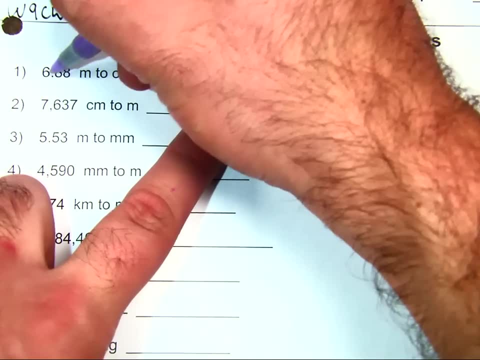 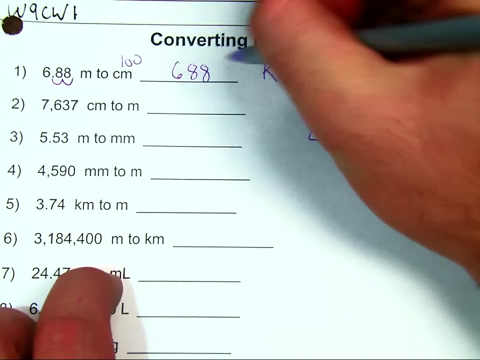 In this case, I'm going to move over two spaces to the right as well, Going one, two spaces to the right. So my final answer will be 688.. I'm going to be doing it in block time. My next one: I'm doing it in block time. 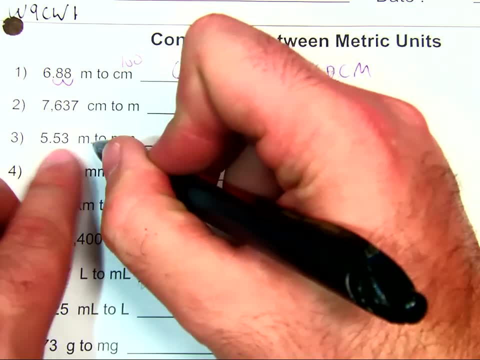 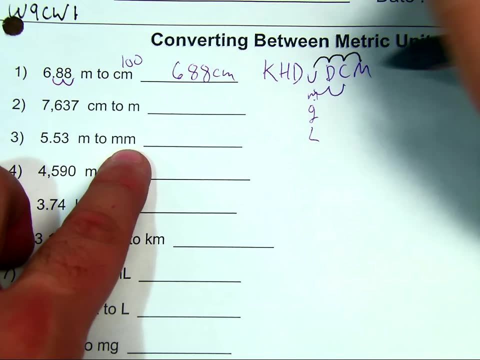 For my next one, I'm going- let's do number three- meters to millimeters. I'm going from my unit, my M, to my millimeter. I'm going one, two, three spaces to the right. So I'm going to go one, two, three spaces to the right. 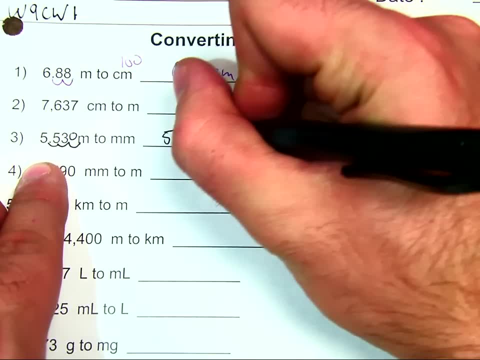 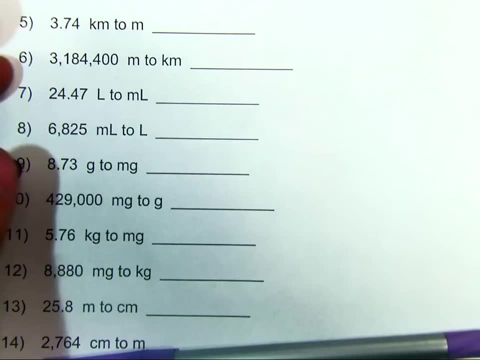 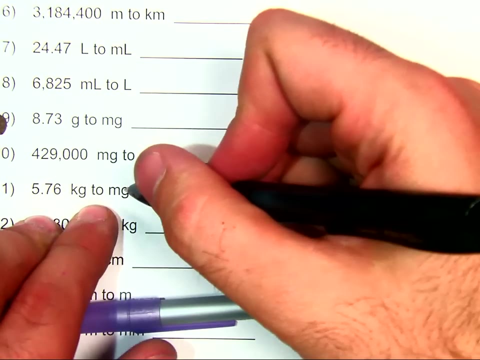 Now I ran out of space, so I have to add a placeholder: 0,, 5530 millimeters. Now what if I have something that's kind of ridiculous, like number 11?? I have 5.76 kilograms to milligrams. 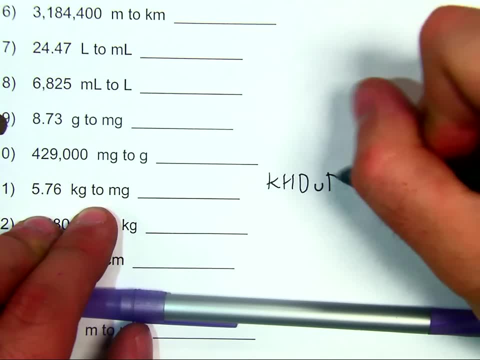 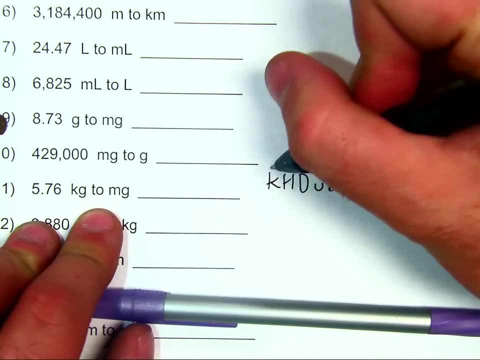 I have. King Henry died unexpectedly drinking chocolate milk. I'm going to go from kilograms all the way to milligrams over here, So I'm going 1,, 2,, 3,, 4,, 5,, 6 spaces to the right. 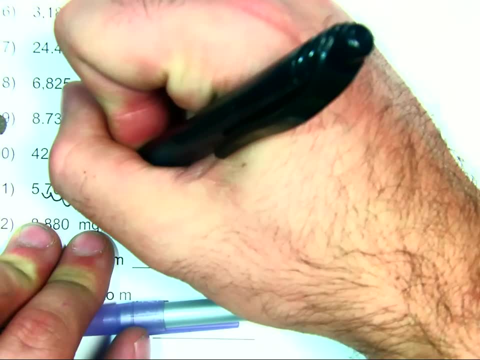 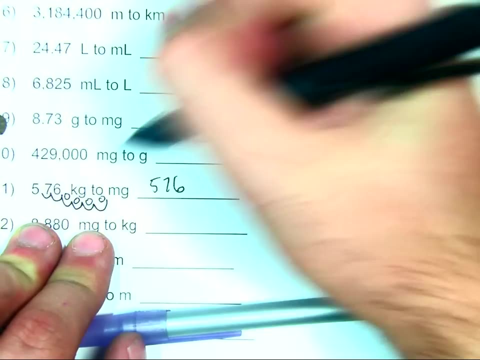 So I'm going to go 1,, 2,, 3,, 4,, 5, 6 spaces to the right- I have 576, and then 1,, 2,, 3,, 4 placeholder zeros. Now I add some commas to make sure it looks right. 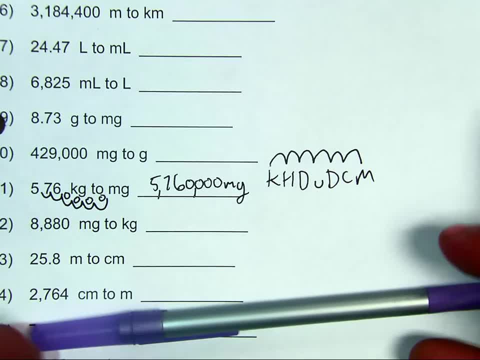 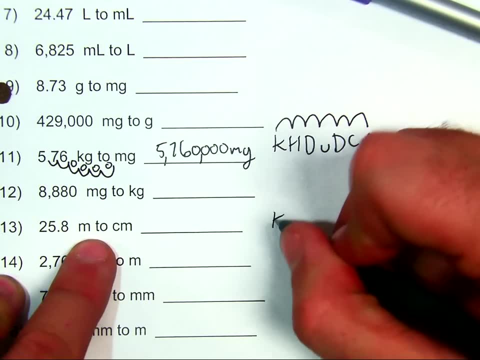 5,760,000 milligrams. And one more. Let's just do our meters to centimeters right here, number 13.. 25.8 meters to centimeters. King Henry died unexpectedly drinking chocolate milk. I'm going: Meters is my unit to centimeters. 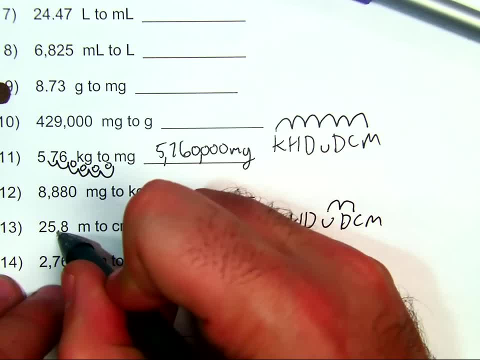 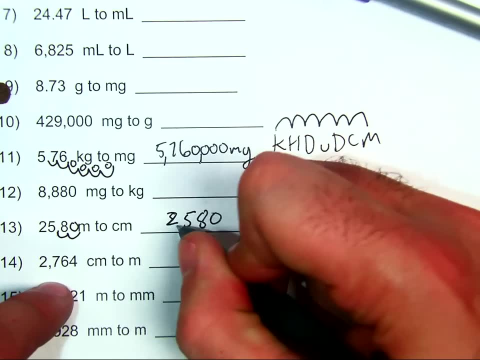 I'm going 1, 2 to the right, So I go 1, 2 to the right. I don't have anything there, so I have to add a placeholder: zero 2,580 centimeters. It makes total sense because there are more centimeters than meters.